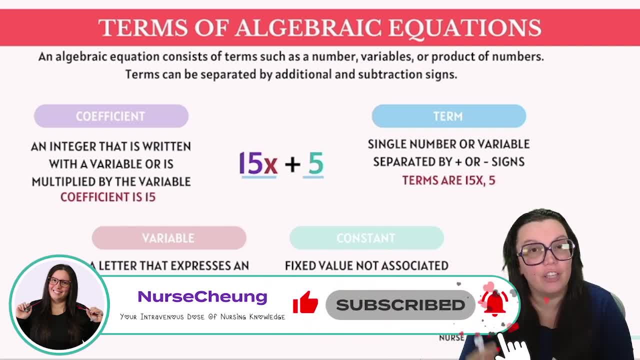 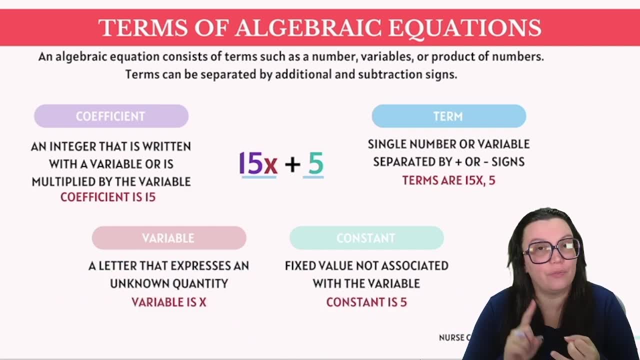 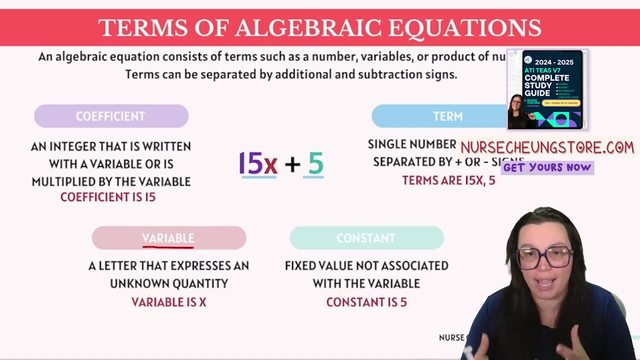 algebraic expression: 15x plus 5.. There are going to be four key terms that are consistently going to be used when you're taking your test. It's going to be coefficient, variable, term and constant. So let's begin with the term variable. So variables are elements within an expression. 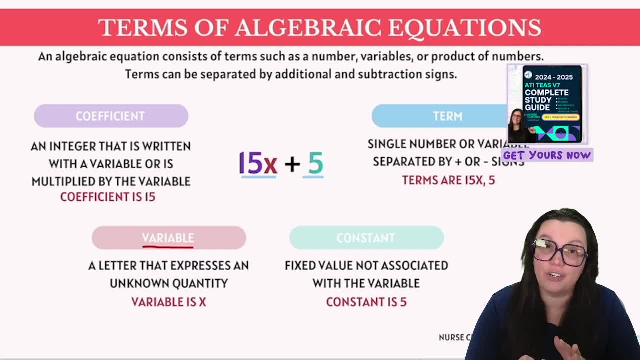 whose values are not fixed. They represent letters of unknown quantities. In our given example that we have here, the one variable we have, x, represents the quantities that are not immediately known without needing additional information. Next up we have our constant. So in our example, 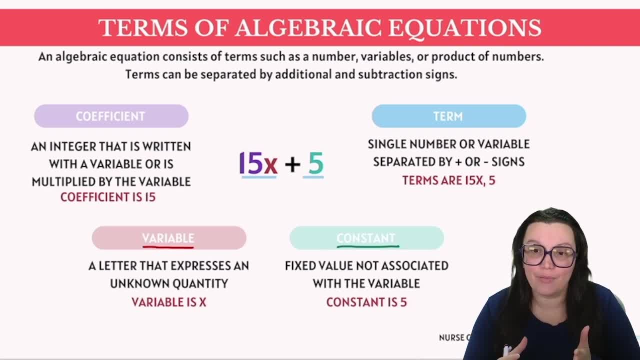 the constant is the number that is represented by the number 5.. It's labeled as a constant because it stands alone without any variable attached to it. Unlike variables whose values might change depending on specific conditions or inputs, a constant remains the same within the expression. Therefore, any number that appears by itself. 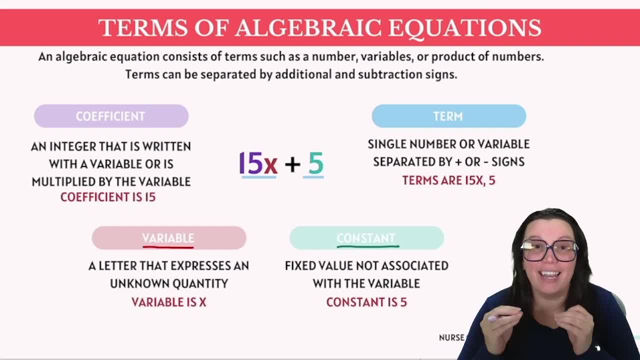 not accompanied by a variable is considered a constant in algebraic expressions. Next up, we have coefficient, and a coefficient is a number that multiplies by a document variable within the expression. So, for instance, in our example our coefficient is actually 15.. 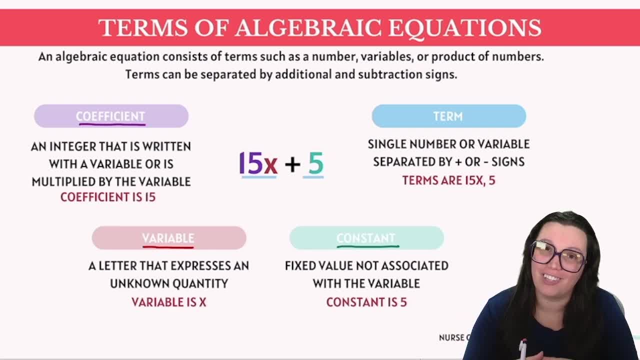 Coefficients and variables are paired together in multiplication relationships And when they are written, that number, our coefficient, always precedes the variable. And finally, let's talk about terms. So in an algebraic expression, a term refers to a component that is delineated. 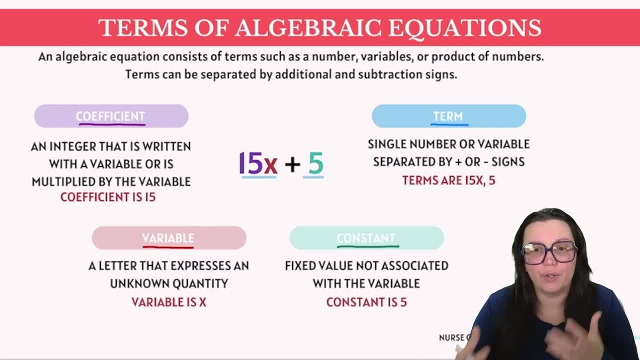 by addition or subtraction symbols. So, for example, in our expression, 15x and 5 each represent distinct terms. So, essentially, terms are the building blocks of an algebraic expression, excluding the operators, that is, our addition and subtraction themselves. Although the concept of 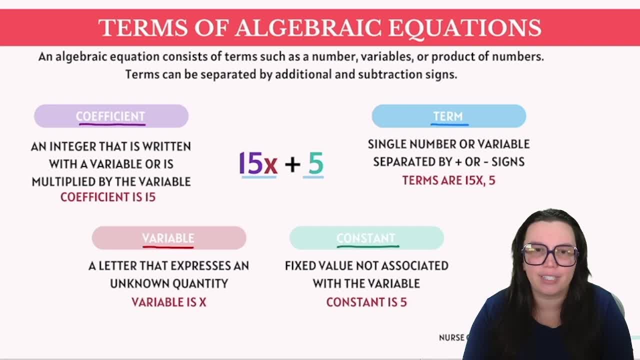 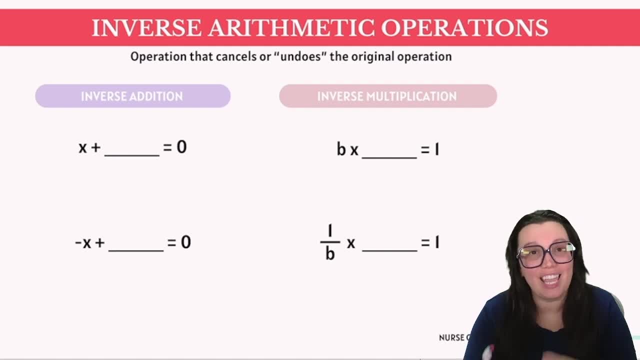 terms might not be the primary focus. it's crucial to understand because it underpins the structure of algebraic expressions. Another important thing to remember is that terms are not always the primary focus of an algebraic expression. Another important concept that you're going to need to know is inverse arithmetic operations. 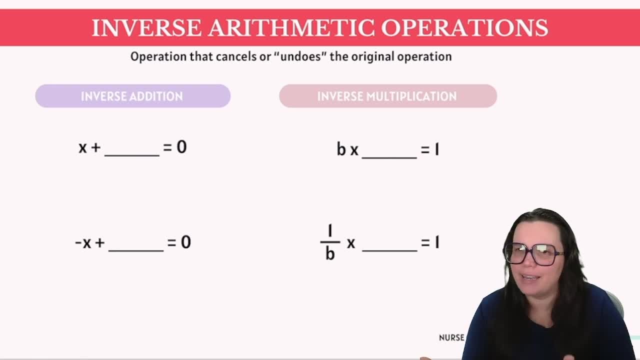 So this principle revolves around the question: what do we add, subtract, multiply or divide into a number for it to result in zero? To illustrate this concept, consider an example where we're looking to find what can be added to a positive number in order to result in zero. 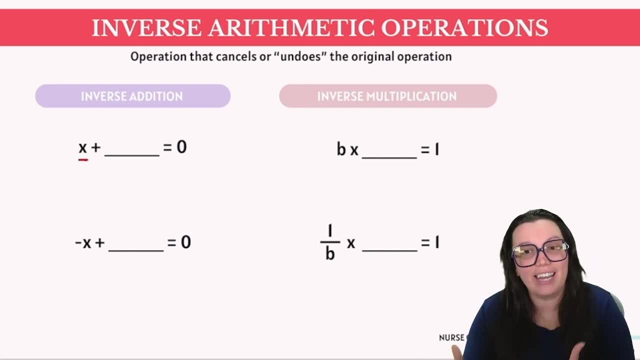 Given that x is a positive number, the additive inverse would be negative x. It's negative counterpoint. Therefore, if you add x to negative x, you're going to get zero. They essentially cancel each other out. In our next example we're dealing with a negative value: negative x To find. 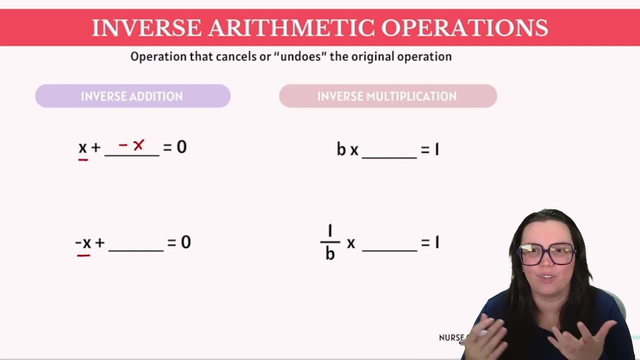 what needs to be added to achieve zero. we use that additive inverse concept, meaning that we need to add the opposite. So negative x plus positive x is going to equal zero, demonstrating the inverse property of addition. Not too bad right. Now let's dive into the next example. 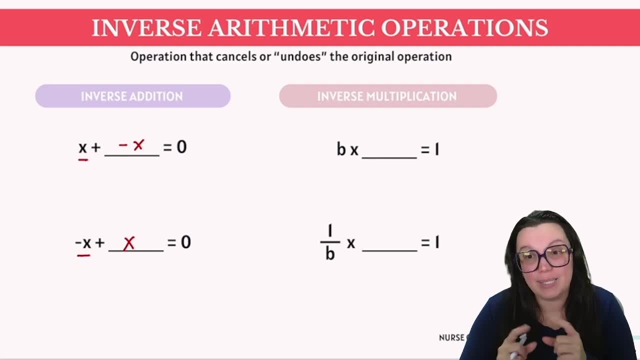 Let's dive into inverse property of multiplication. This principle is centered around identifying what number, when multiplied by another, is going to yield one. Essentially, any number times its multiplicative, inverse or reciprocal equals one. So for our first example, consider the letter B, where B is a whole number and not a fraction. It's actually quite helpful to represent. 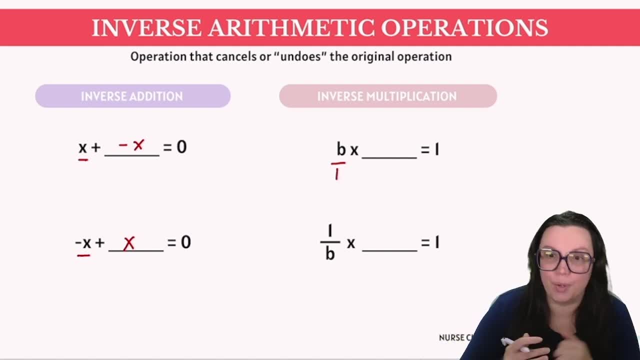 B in its fractional form, as B over one, where B is a whole number and not a fraction. Any whole number can be expressed as a fraction over one. To find the reciprocal, we invert the fraction, making the denominator the new numerator and the numerator the new denominator. Therefore, 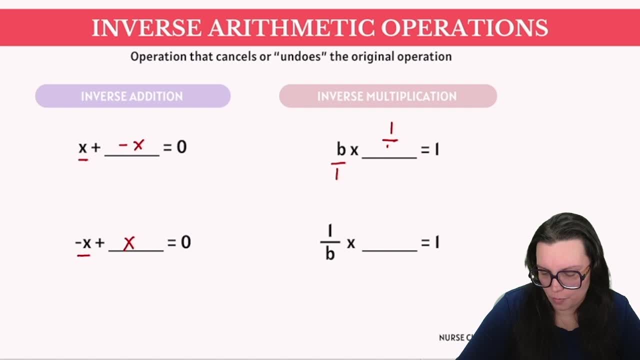 the reciprocal of B is actually one over B. To verify this, let's multiply B in its fractional form as B over one by its reciprocal one over B. When multiplying fractions, we multiply the numerators together and the denominators together. Starting with our numerator, we have B times one is going to give us B And with our denominators, 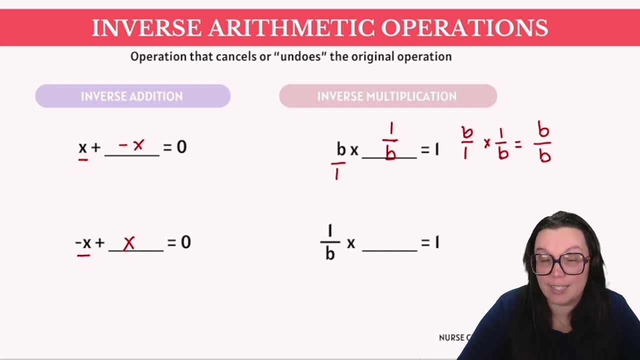 we have one times B is also going to give us B. This is ultimately going to give us B over B, which further simplifies into the number one. We may also encounter a fraction of one over B. In order to identify the reciprocal, we simply flip the fraction, resulting in B over one. 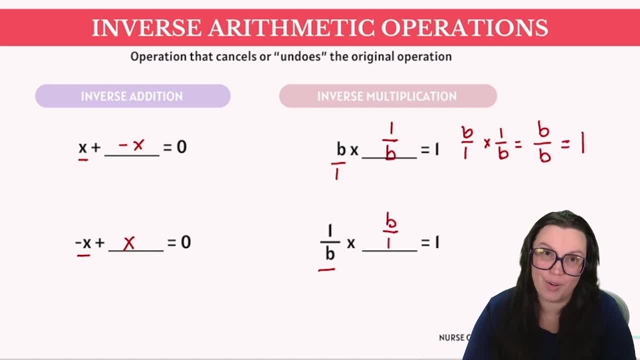 And, just like we did in our previous example, when we multiply our numerators and our denominators, we simplify it to B, or that's also going to equal one. Let's take a look at some examples for solving equations using one variable. So when we're performing these operations, we want to 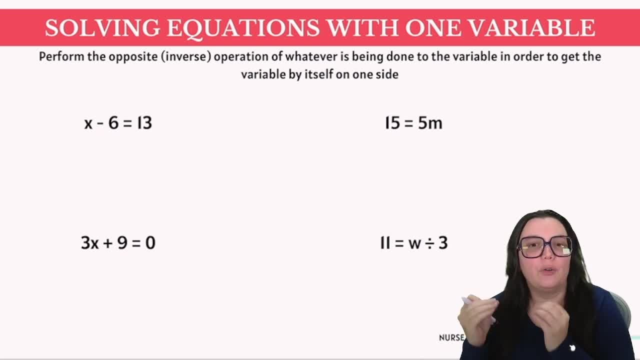 perform the opposite or inverse operation of whatever we are doing on one side of the variable to the other side of our equation. So our first example: we have X minus six equals 13.. So we want to isolate X in order to find out what that number is. So what we're going to do is just like: 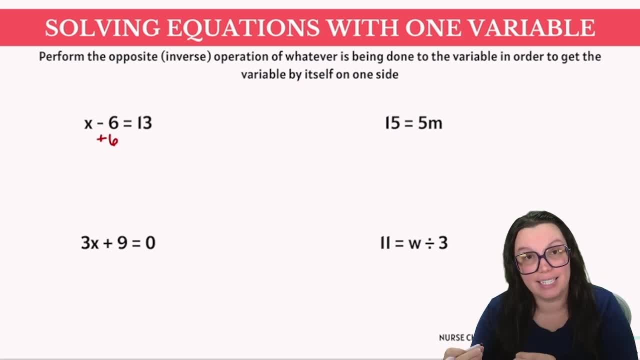 before. we're going to do the inverse. So we have a negative six. We're going to add a positive six to both sides. Adding a positive six is going to give us X equals 19.. We just solved our first equation And our next example. we have three X plus nine equals zero. So again we want to isolate. 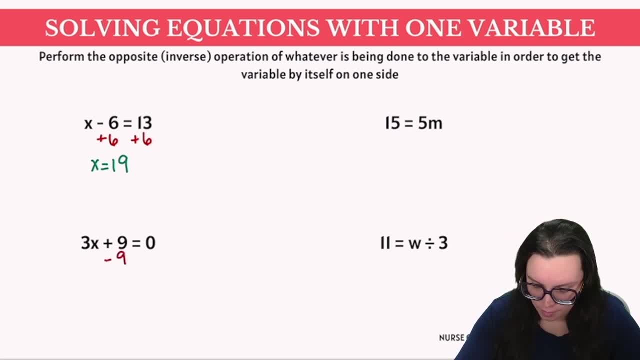 X first. So we do that by minusing nine from both sides, because here we had a positive nine. We want to make sure that we minus nine in order to achieve zero. Once we do that, we're going to get three. X is equal to negative nine, And now we need to again. 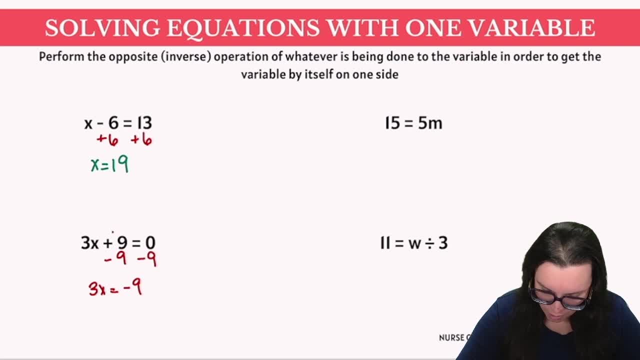 isolate that X. So how are we going to do that? We are going to go ahead and divide by three on both sides in order to get rid of that three coefficient before our variable That is going to give us X is equal to negative three. Our next example: we have 15 equals five M. So 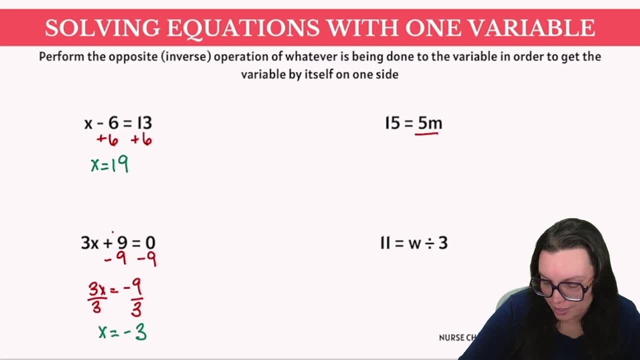 again, we want to isolate that variable. That's our M. So we're going to divide five by both sides And that is going to give us three is equal to M. And our last example may seem a little bit tricky, but actually it's really quite simple. We have: 11 is equal to W divided by three. So again, 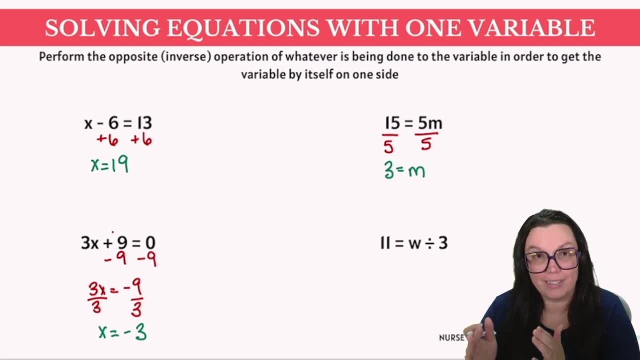 we want to isolate our variable. We want to get that W on one side by itself. In order to do that, we're going to multiply each side by three, because that is the inverse operation And that is going to give us: 33 is equal to W. Not too bad right? So next up. 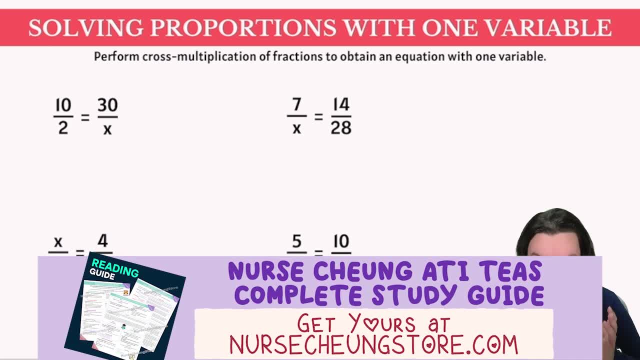 we're going to solve proportions with one variable. So you're going to see two fractions with an equal sign between them and you're going to have to solve for whatever the variable is, whether it's X or another letter. So in order to do this, we're going to cross, multiply fractions to obtain an. 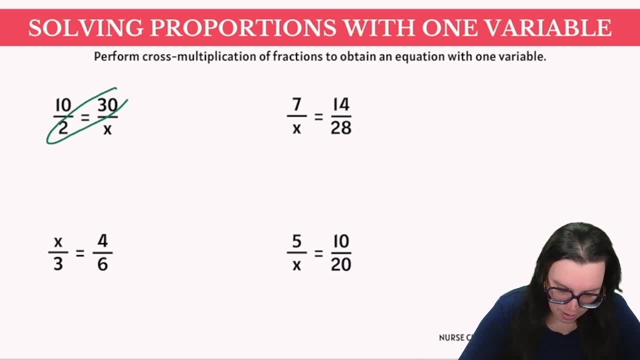 equation with one variable. So we do this by cross multiplication of our fractions and that is going to give us 10X is equal to 60.. So now we have an algebraic expression and we just need to solve for X. So we do so by dividing each side by 10,. 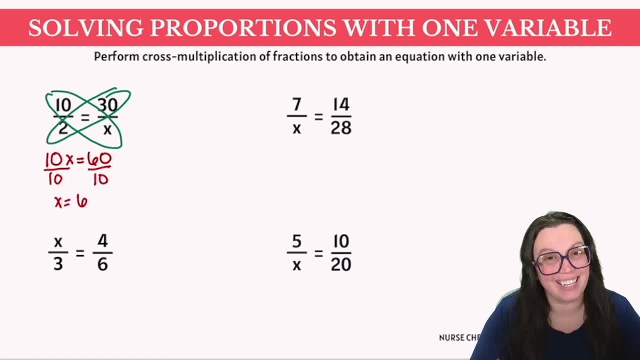 and that is going to give us X is equal to six. Let's try another example. So down here we have: X over three is equal to four over six. So again, we are going to cross, multiply our fractions and that is going to give us six. So we're going to cross, multiply our fractions. 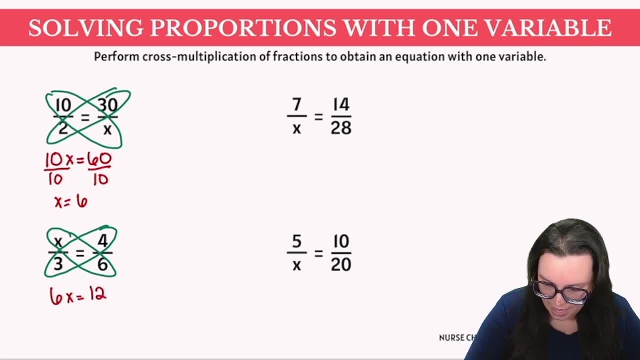 and that is going to give us that is equal to 6X. So now let's go over to our first equation. Let's say that we have I, or even more graceful, good nebulous, and that we're going to convert that each step into six. So we can then go ahead and say: let's divide this into 14.. So again, 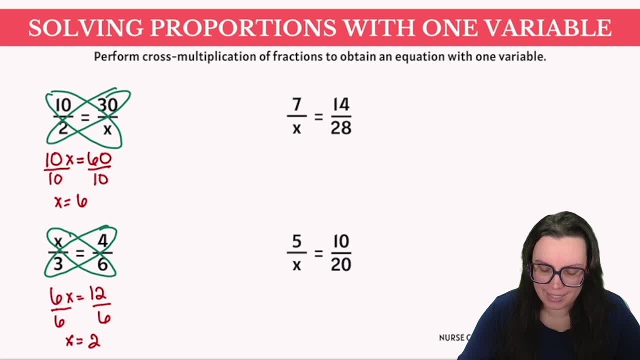 we're going to be putting it over there, but it's lowercase square, so it's x plus 14x. but we're going to start here, We're going to split it into everything And then we're going to double that. over and over, C is equal to one. 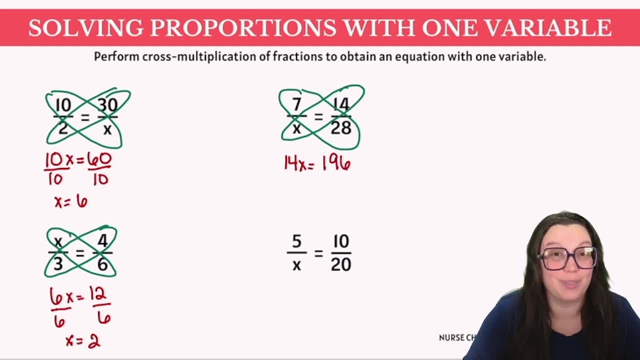 five, and then we multiply our fractions, so that's going to give us 100x. So now that is to 96.. We're dealing with big numbers. now, right, We are again going to isolate our x by dividing each side by 14.. And that is going to give us our correct answer of x is equal to 14.. Hopefully this. 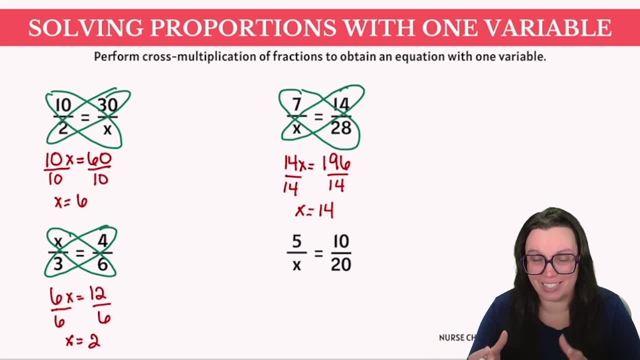 has helped bridging some gaps in understanding how we cross multiply proportions. So let's move on to our final example. So we have 5x. 5 over x is equal to 10 over 20.. So we're going to go ahead. 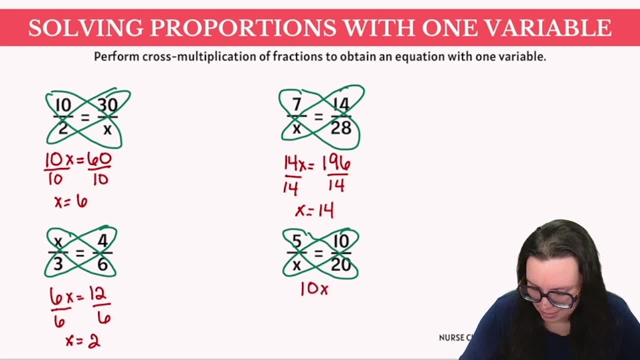 and cross multiply. This is going to give us 10x is equal to 100. And, of course, we're going to divide each side by 10 in order to isolate x, And that is going to give us our final example of x. 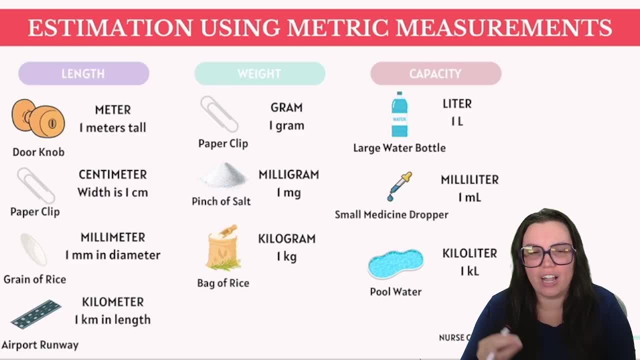 is equal to 10.. So let's talk about estimation On the ATATs. you're going to have to use your best judgment in regards to length, weight and capacity when it comes to various items. So, starting with the estimation involving length, you're going to 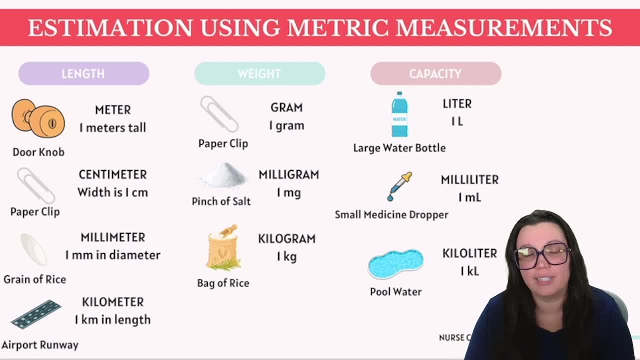 be using metric system conversions. It is a crucial skill that you're going to need to know for the ATATs as well as healthcare, So choosing the appropriate unit of measurement depends on the object that you are measuring. If you haven't already done so, I highly recommend that you go. 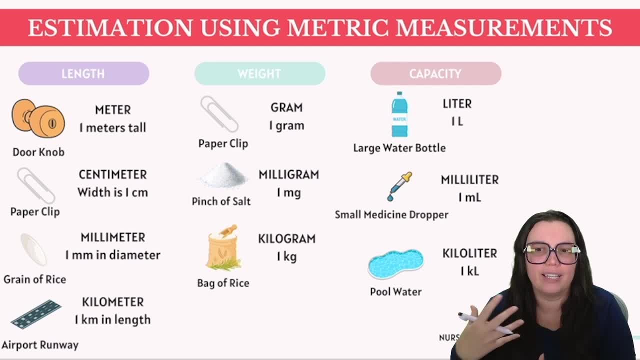 check out my video on metric conversions, because it's going to help you break down the differences between each unit and how we establish each one. But let's take a look at how the ATATs is going to test you when it comes to this. So, when it comes to length, there's a couple different things. 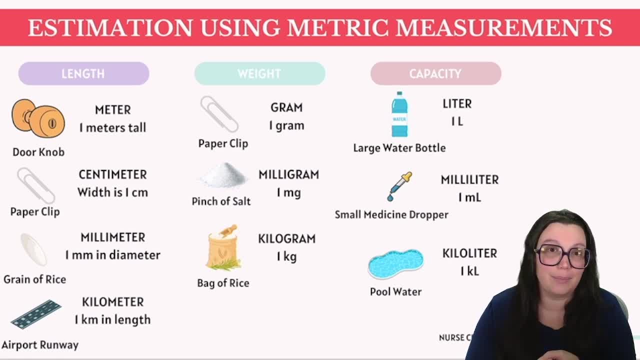 that you can do, So let's take a look at how the ATATs is going to test you when it comes to this. You're going to need to know meter, centimeter, millimeter and kilometer. So, starting with the, 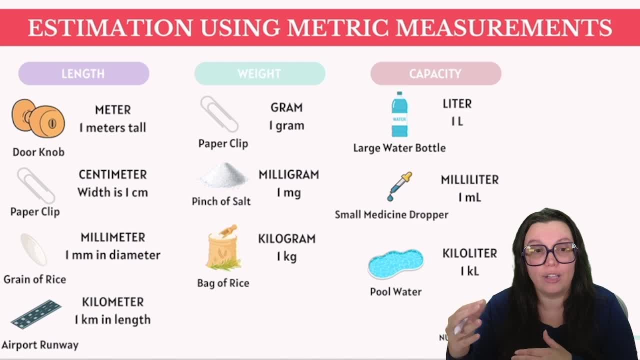 meter. just to give you real life examples, one meter tall is about the height of a doorknob. So when you look at your doorknob, that is about the height of one meter. When we're talking about centimeter, we're talking about the width of a paper clip. That's approximately one centimeter. 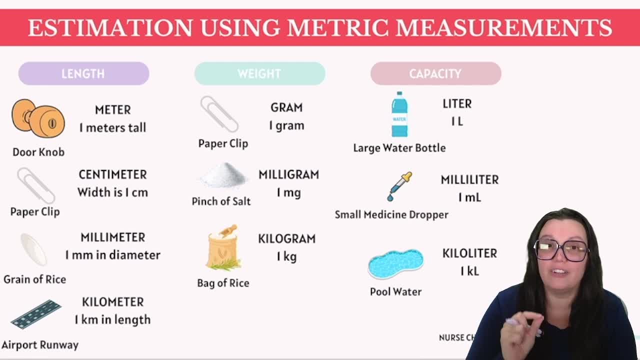 When we're talking about millimeter, that is, approximately one millimeter, is the diameter of a grain of salt. So when we're talking about millimeter, that is, approximately one millimeter, It's really, really, really, really tiny. It's not the length of the grain of salt, It's that. 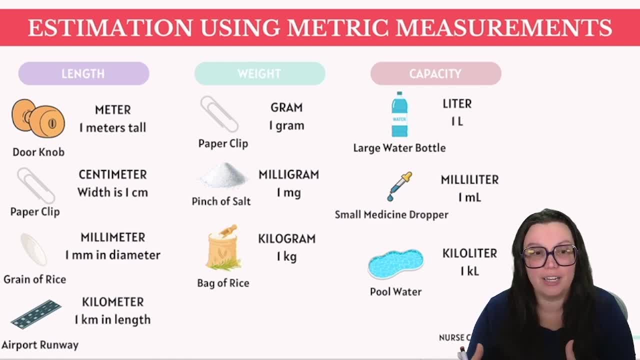 diameter that cut through. And then, lastly, with kilometer. when we think of kilometer, one kilometer is equal to an airport runway. So if you've ever been in an airplane, you know that runway is very long. That is approximately one kilometer. Next up we have weight, So 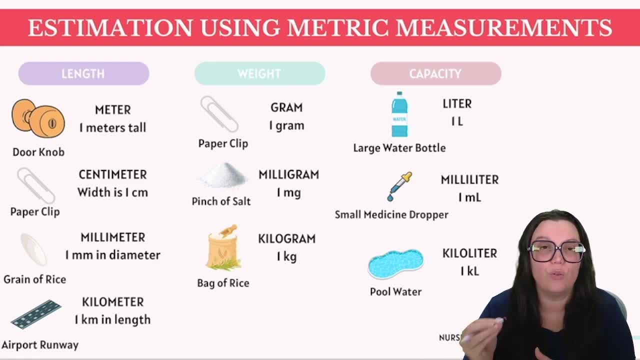 approximately. when it comes to weight, a gram is equal to the weight of a paper clip. So that paper clip is not very heavy, right? So it's very, very light. So that's approximately one gram. Next up we have milligram. So one milligram is essentially the same weight as a. 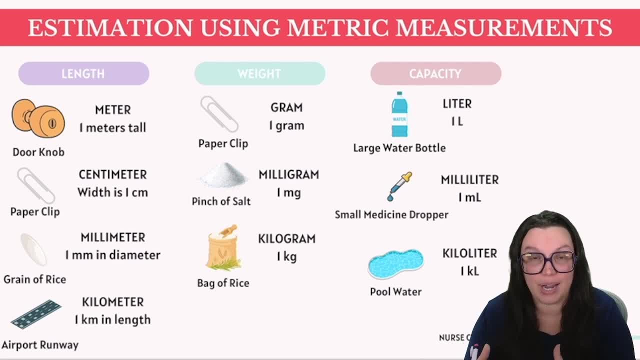 pinch of salt, So not very big. And then lastly, kilogram, So one kilogram is approximately the weight of one bag of rice. And last up we have capacity, So one liter. if you look at those large water bottles, even like this water bottle, right, This water bottle is approximately one liter. 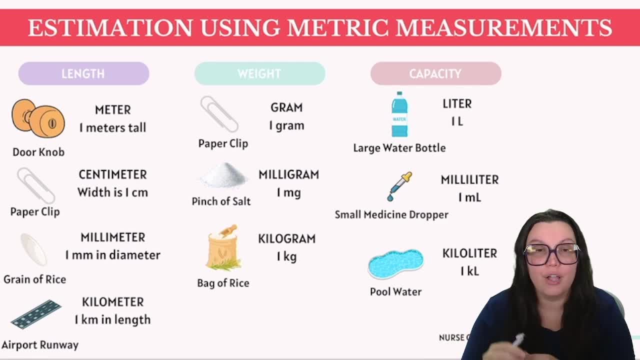 Then we have milliliter, So this is huge in healthcare. So one liter is just like a small medication dropper amount of liquid. And then, lastly, we have a kiloliter, So a kiloliter is approximately the entire capacity of a pool of water. So let's take 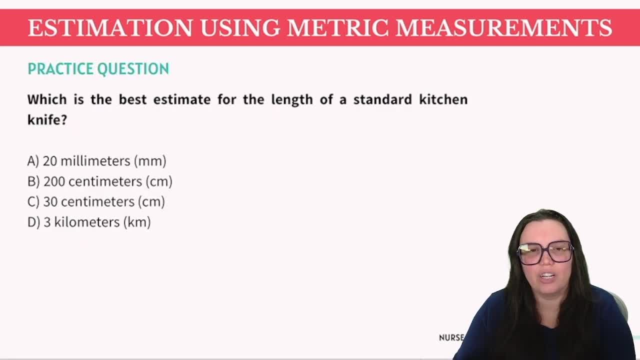 a look at some examples of how this will be tested on the teas. So, starting with question one, what is the best estimate for a length of a standard kitchen knife? So we're talking about the length, So is it 20 millimeters, 200 centimeters, 30 centimeters? 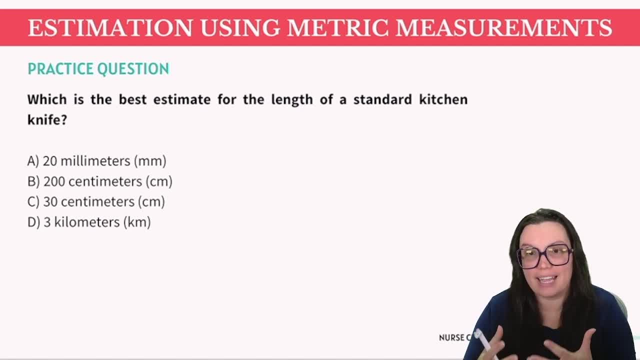 or three kilometers. So, taking a look back at our examples, we know that a standard kitchen knife is not going to be as small as 20 millimeters. right, That's that diameter of our grain of rice, So we can automatically eliminate A, And it's definitely not as long as 200. 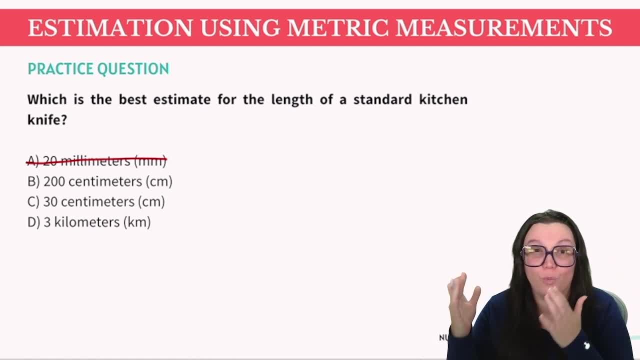 centimeters. Think about it: 200 paperclips width, That's way too long, So we can automatically eliminate that as well. And then, of course, three kilometers, that would be three airport ways. So we definitely know that that is also not our correct answer. So out of all the ones that we 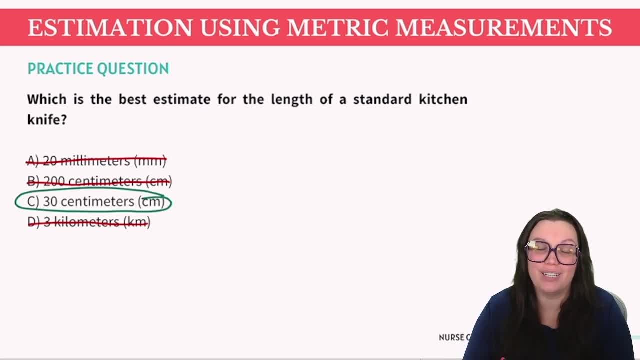 have available to us, C 30 centimeters is going to be the most correct answer. Our next question is: what is the most appropriate unit and estimate for the weight of a car? Is it A 1,500 grams, B- 1.5 kilograms, C- 1,500 kilograms or D- 15,000 milligrams? 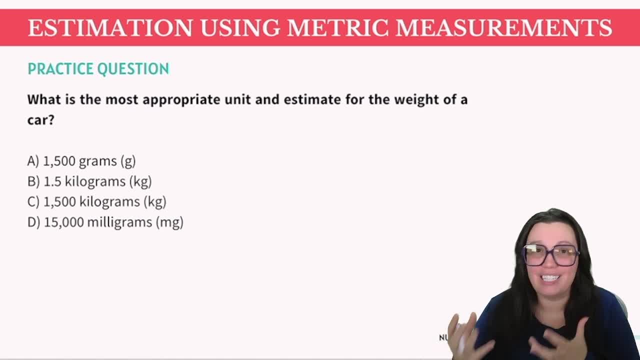 So in order to answer this question, we have to know that cars are significantly heavier than small objects measured in grams and milligrams. So we can automatically eliminate anything that has grams or milligrams from our question. So now we're just left with kilograms.